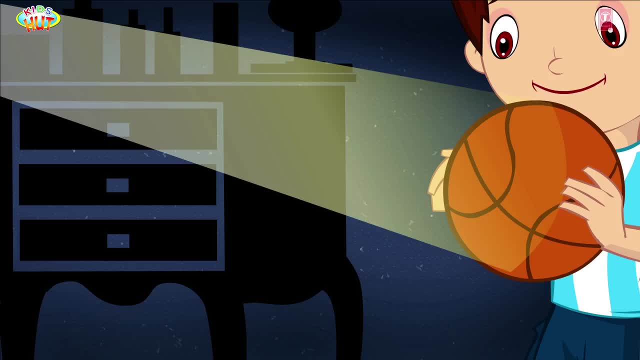 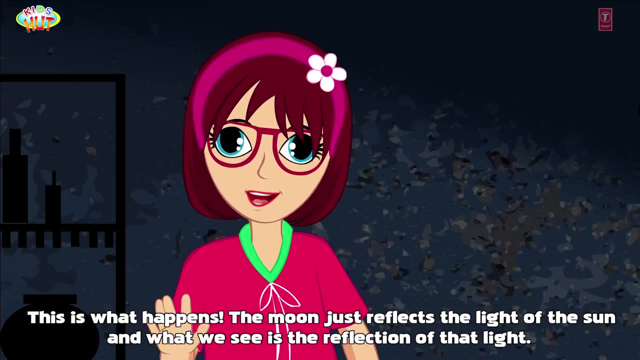 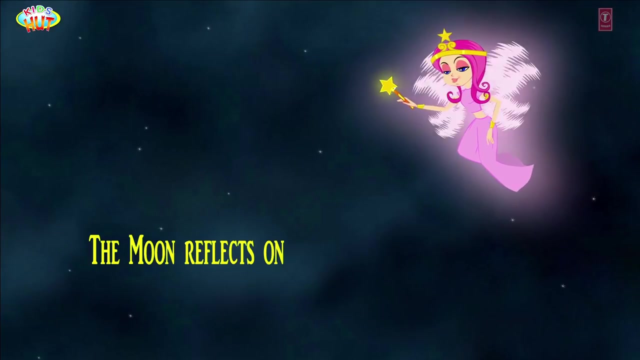 and that light getting reflected on the ball Tofu? Yes, This is what happens. The moon just reflects the light of the sun and what we see is the reflection of that light. Oh Oh, The moon reflects only 7% of the sun's light. 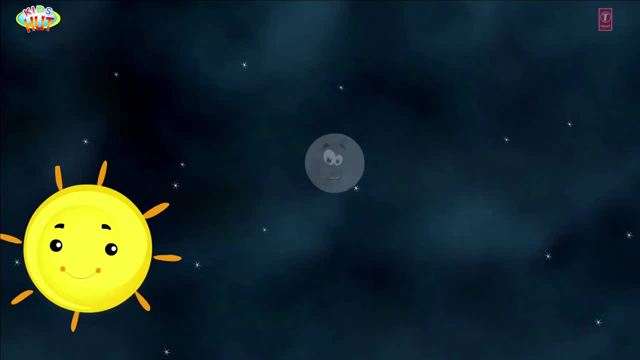 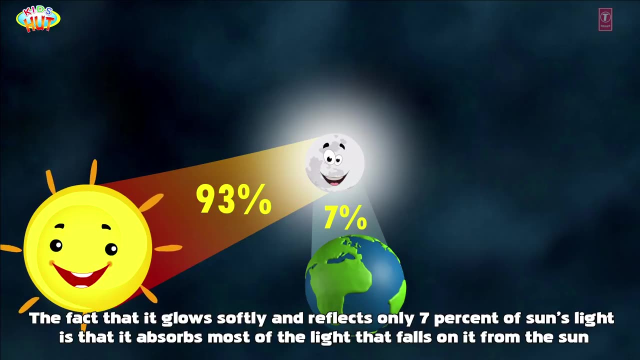 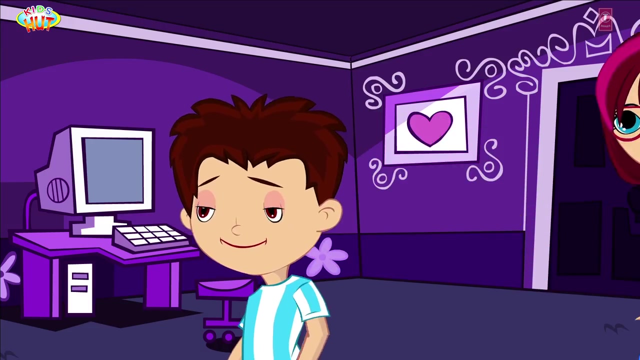 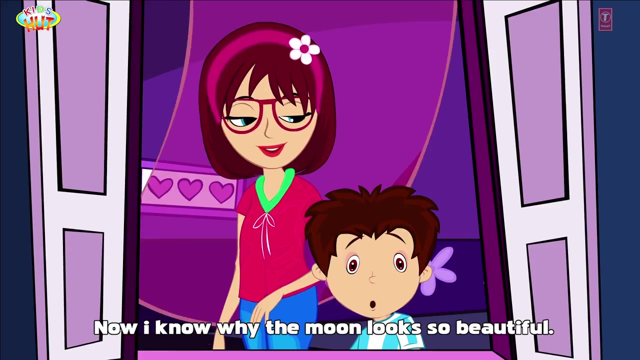 And then it glows softly. The fact that it glows softly and reflects only 7% of the sun's light is that it absorbs most of the light that falls on it from the sun. Now I know why the moon looks so beautiful. 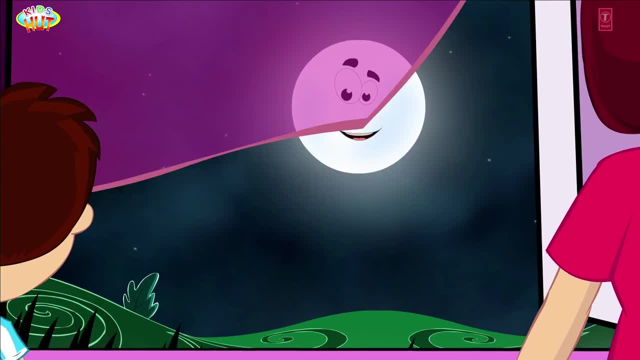 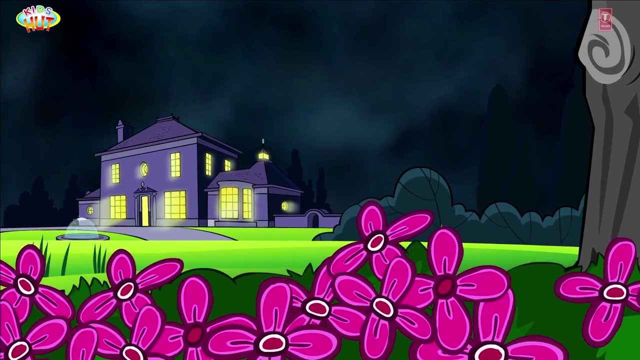 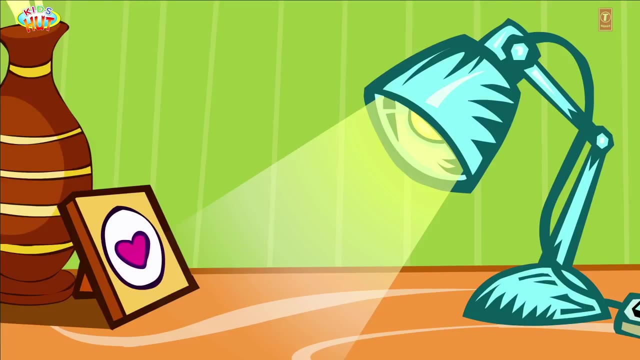 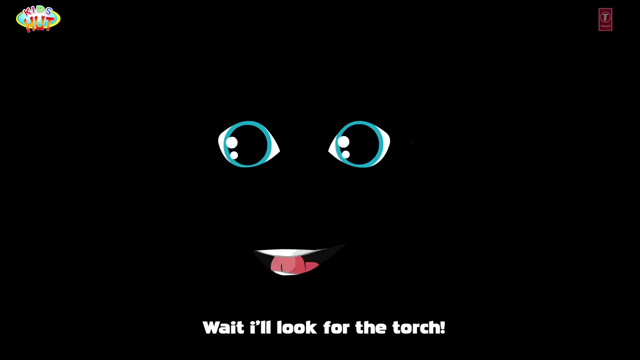 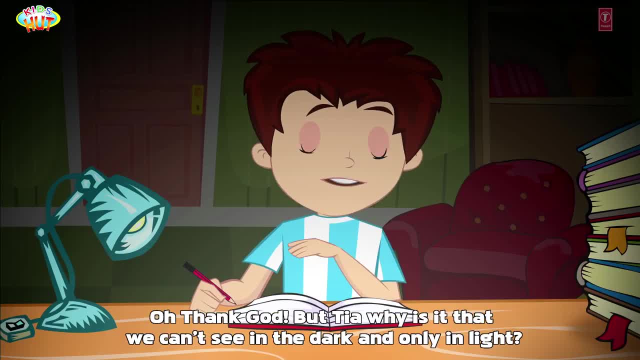 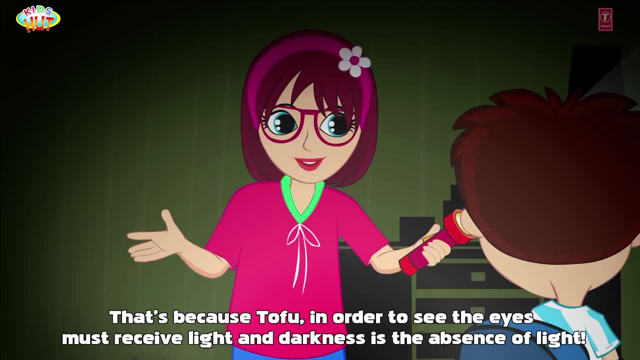 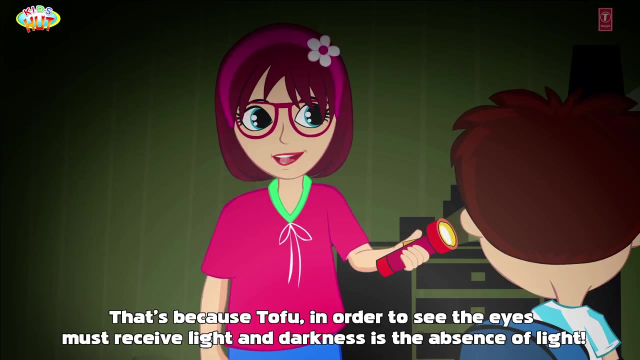 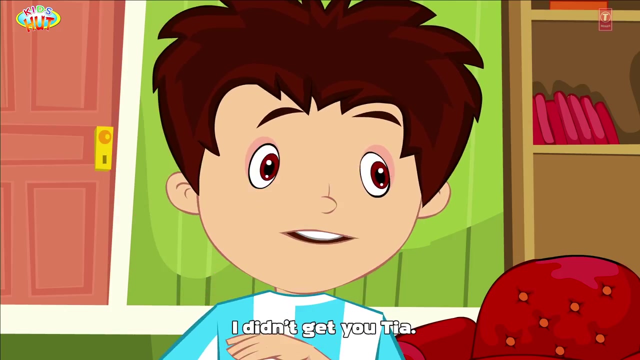 Oh, thank God. But, Tia, why is it that we can't see in the dark and only in light? That's because Tofu, in order to see, the eyes must receive light, and darkness is the absence of light. I didn't get you, Tia. 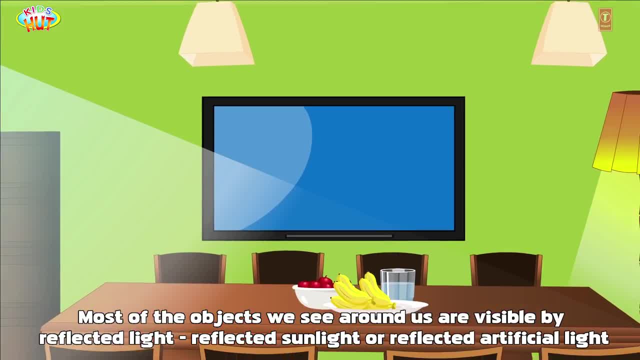 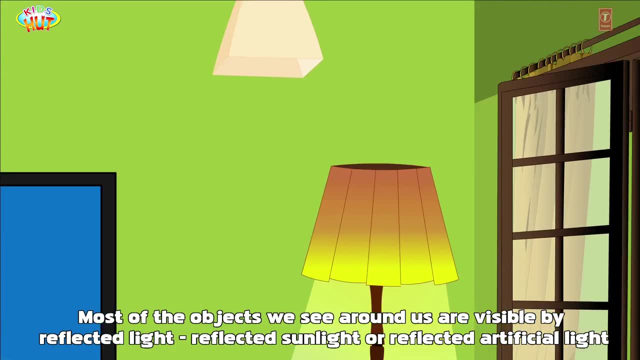 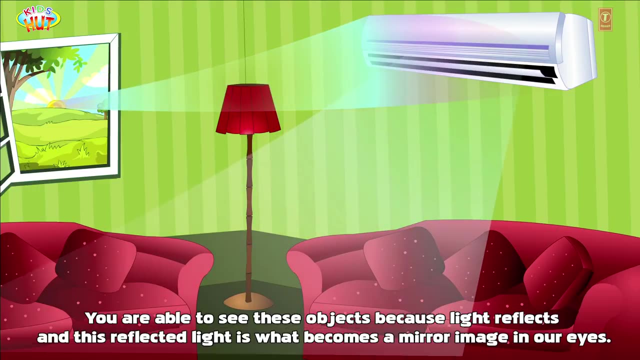 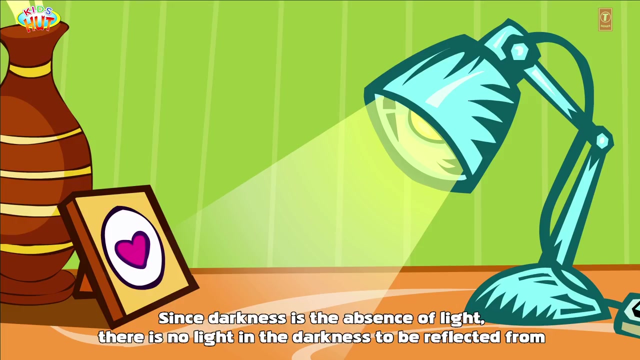 Most of the objects we see around us are visible by reflected light, reflected sunlight or reflected artificial light. You are able to see these objects because light reflects, and this reflected light is what becomes a mirror image in our eyes, Since darkness is the absence of light. 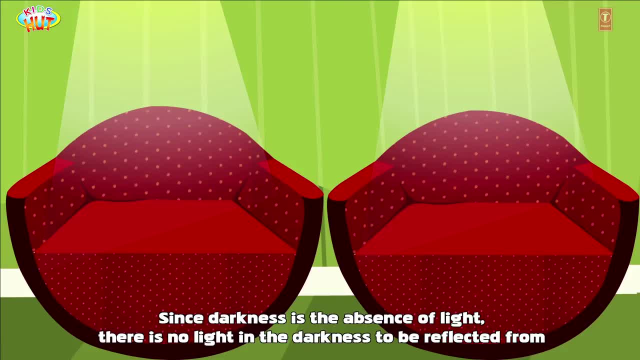 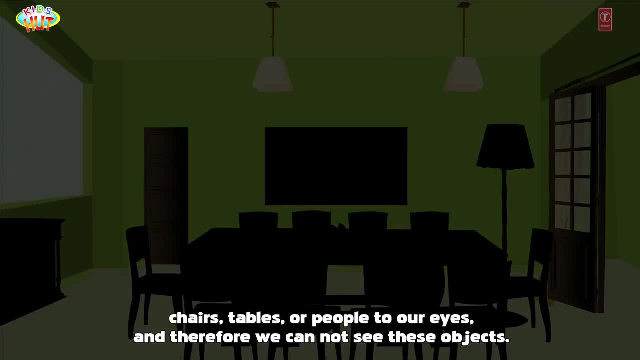 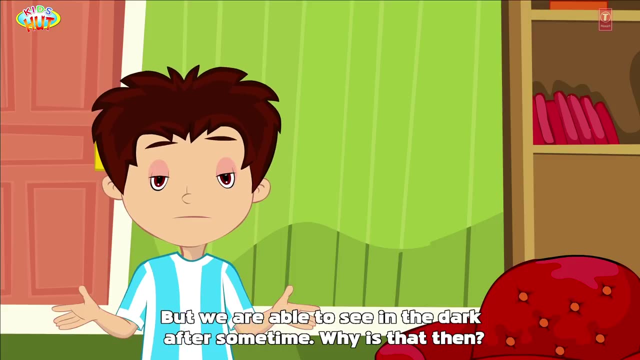 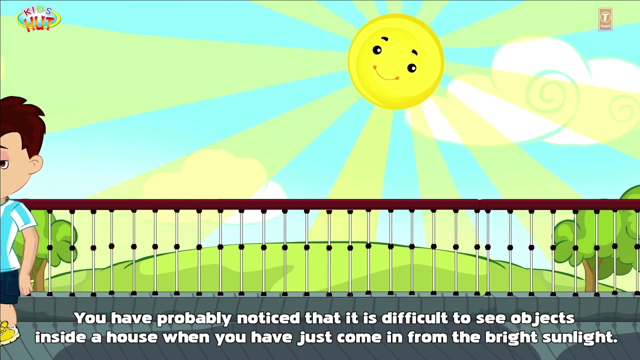 there is no light in the darkness to be reflected from- From chairs, tables or people to our eyes, and therefore we cannot see these objects, But we are able to see in the dark after some time. Why is that then? You have probably noticed that it is difficult to see objects inside a house. 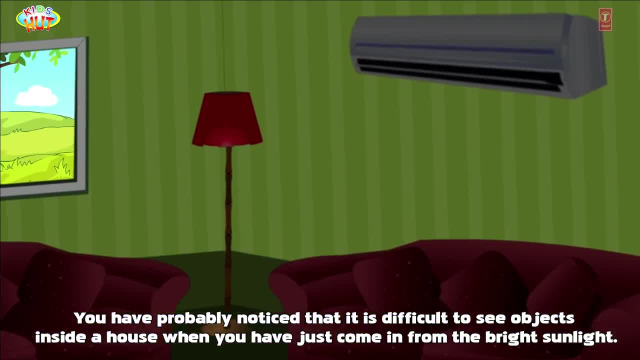 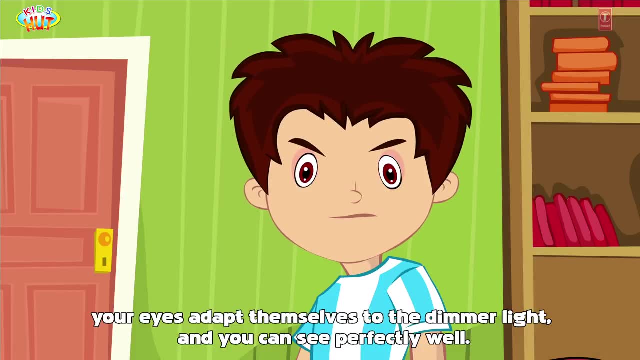 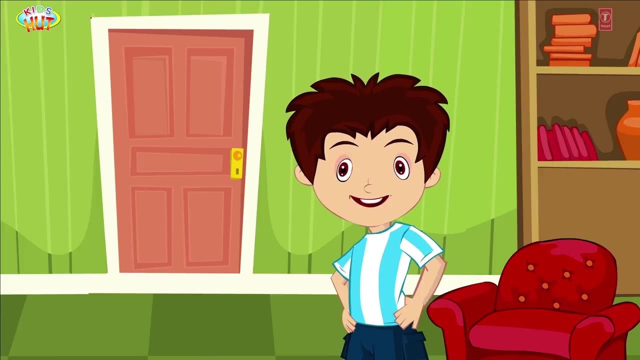 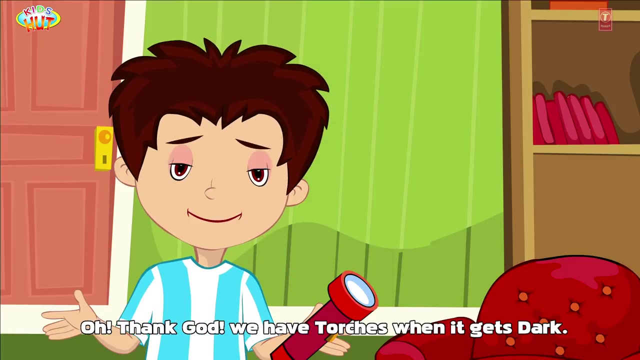 when you have just come in from the bright sunlight, After you have been in the house a little while, your eyes adapt themselves to the dimmer light and you can see perfectly well. Oh, Thank God We have torches when it gets dark. 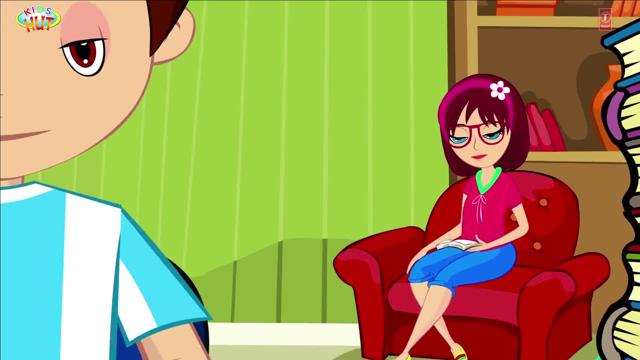 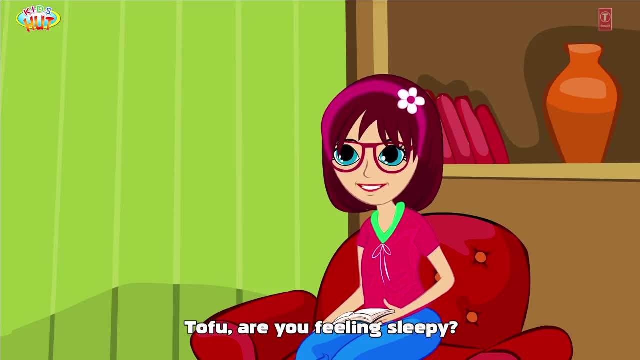 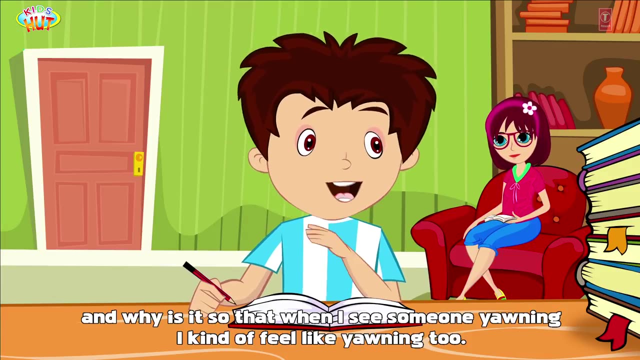 The torches in the house are more beautiful than the lights. This light is the light of the darkness. Tofu, are you feeling sleepy? No, just tired. But Tia, what makes us yawn? And why is it so that when I see someone yawning, 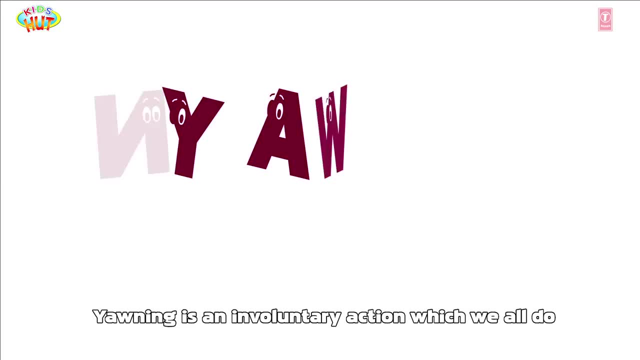 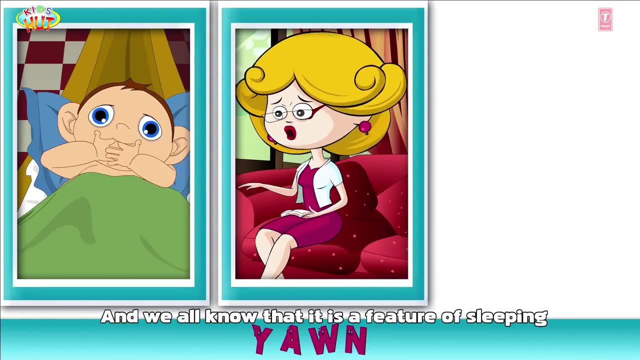 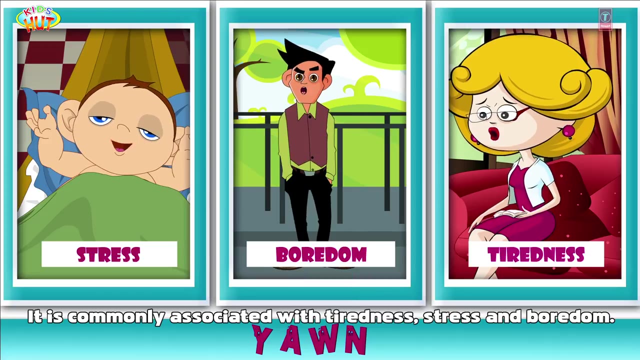 I kind of feel like yawning too. Yawning is an involuntary action which we all do And we all know that it is a feature of sleeping. It is commonly associated with tiredness, stress and boredom. All vertebrates do yawn, including fish and birds. 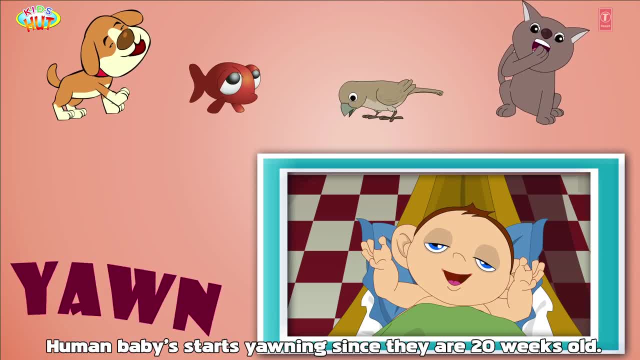 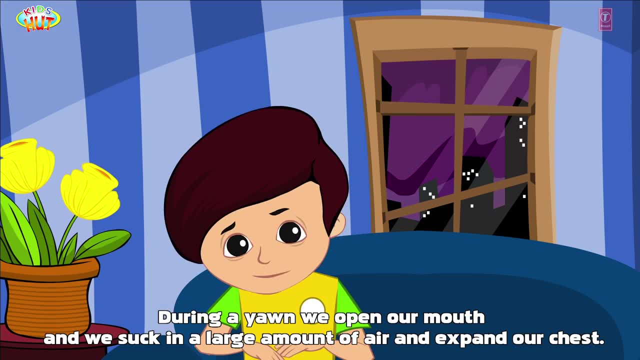 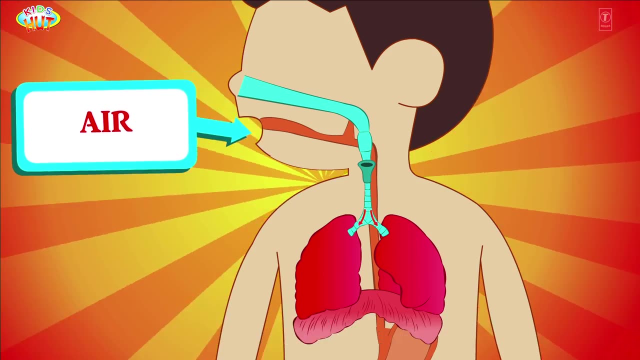 Human baby starts yawning, since they are 20 weeks old. So how do we do it? During a yawn, we open our mouth and we suck in a large amount of air and expand our chest. The cavity pulls down our diaphragm and fills air in our lungs. 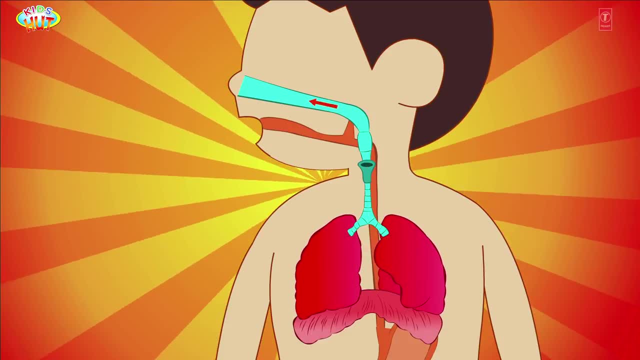 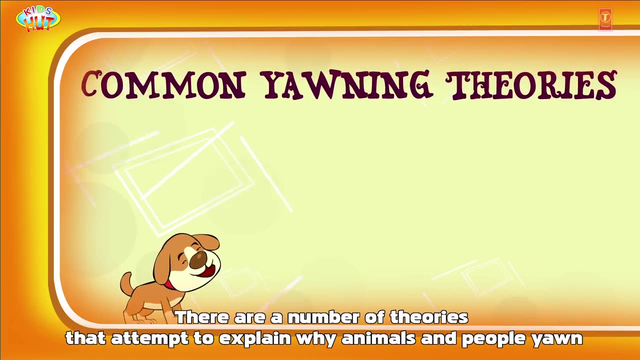 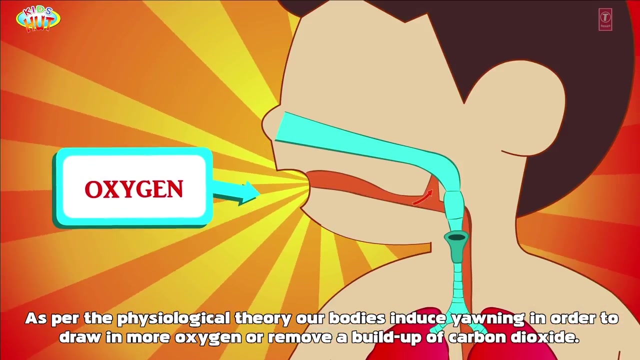 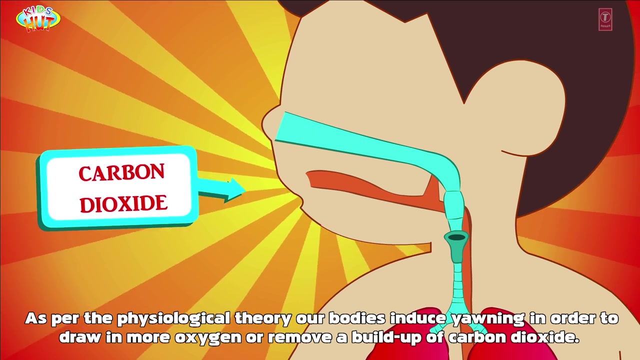 and exhales it out. There are a number of theories that attempt to explain why animals and people yawn. As per the physiological theory, our bodies induce yawning in order to draw in more oxygen or remove a build up of carbon dioxide. A more recent theory explains that we yawn more in the situations. 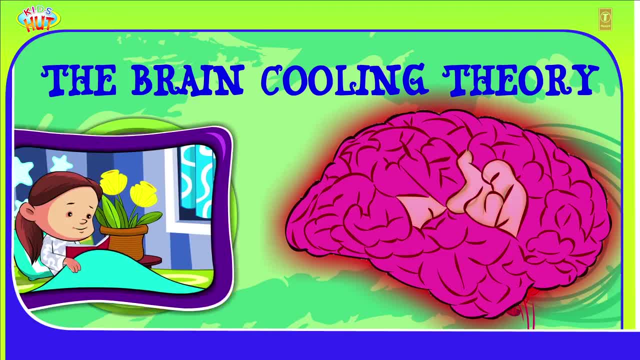 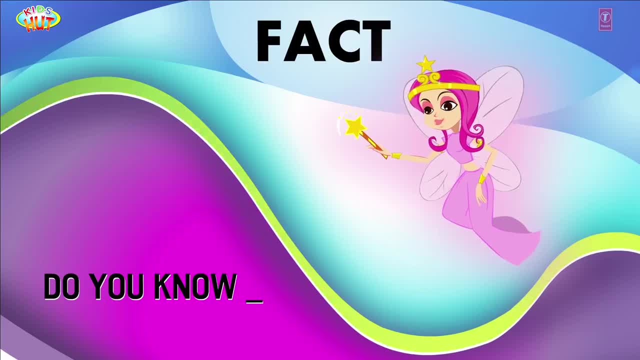 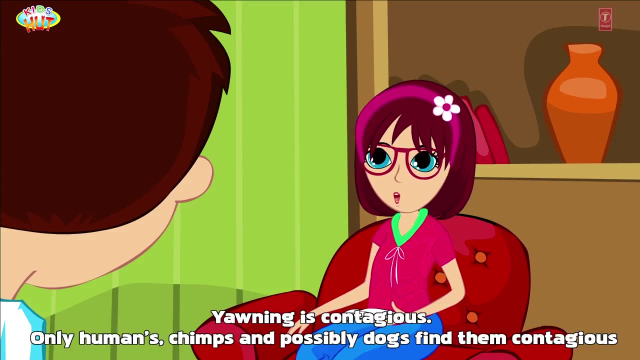 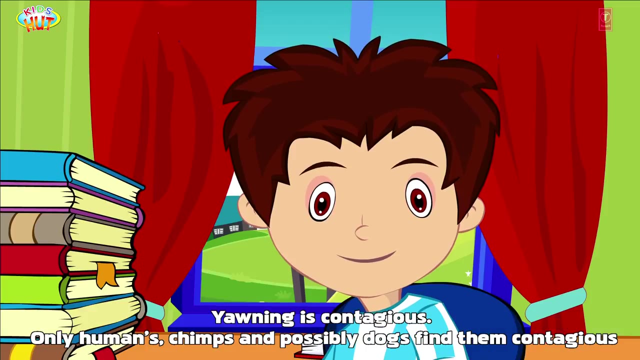 where our brain is likely to be warmer. So it's a way to cool down our brain. Do you know that the average yawn lasts around 6 seconds? Yawning is contagious. Only humans, chimps and possibly dogs find them contagious. 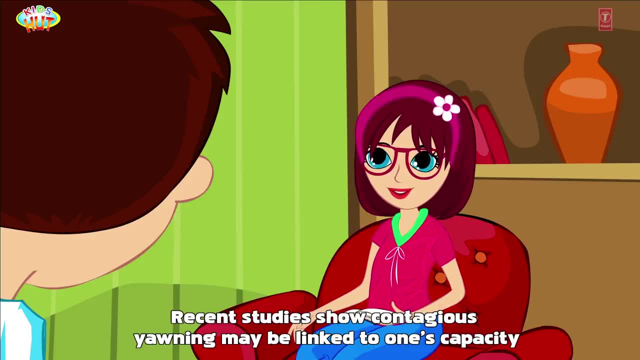 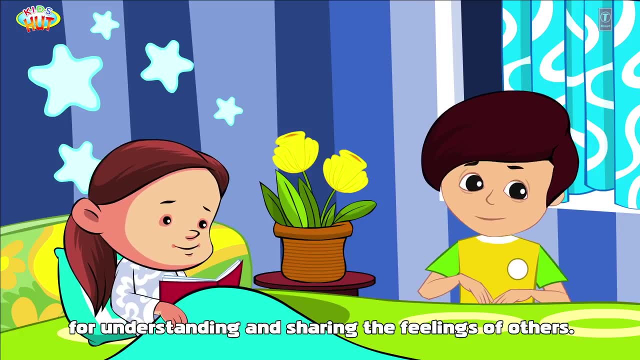 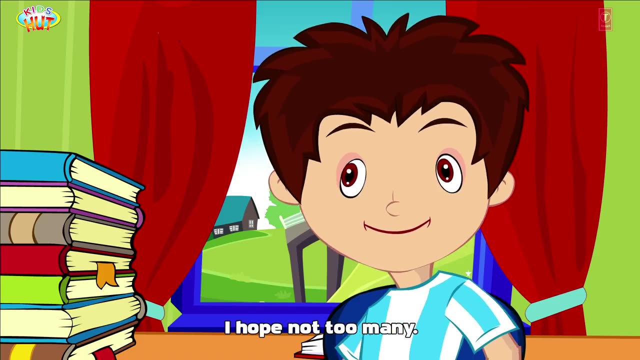 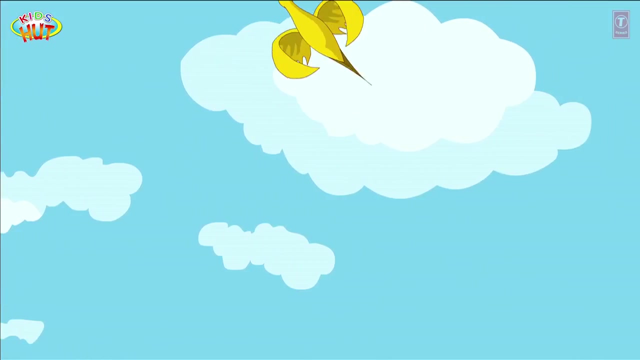 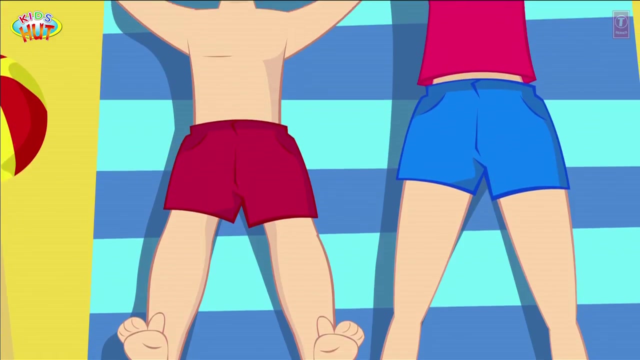 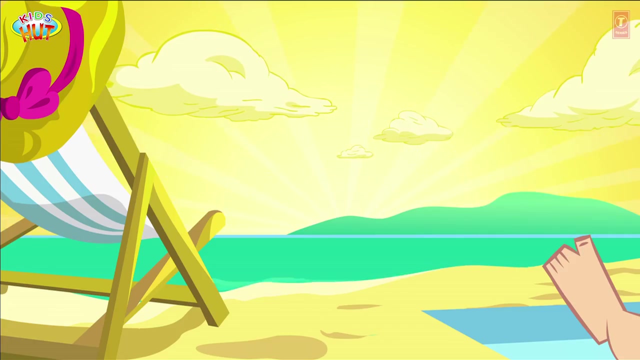 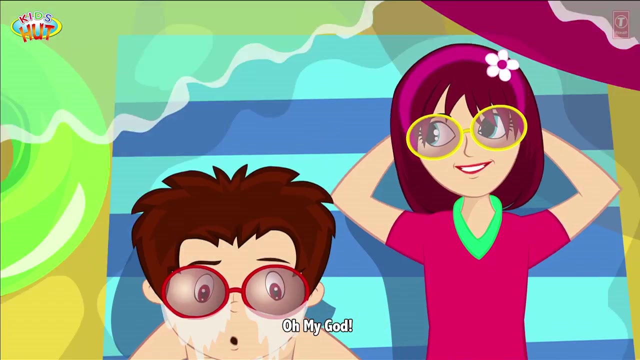 Recent studies show contagious yawning may be linked to one's capacity for understanding and sharing the feelings of others. So, Tofu, how many times have you yawned while listening to me? I hope not too many. Ha ha ha. Oh, my God, this was so much fun. 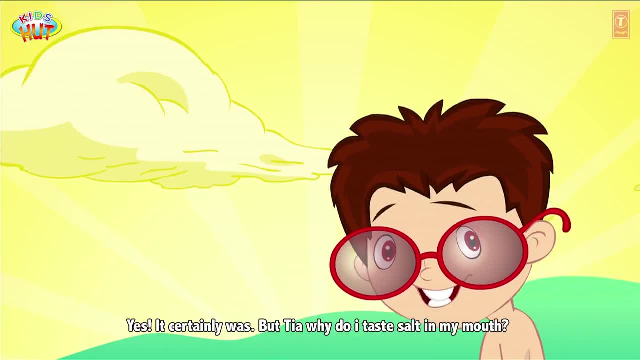 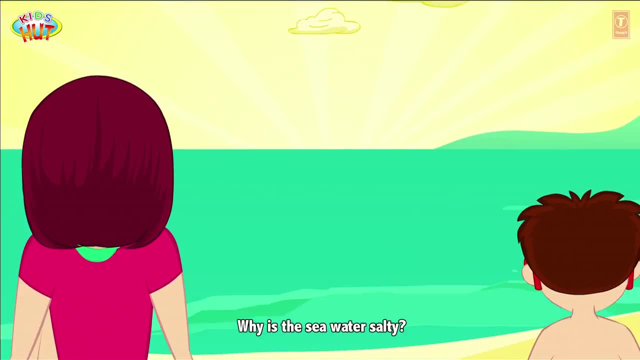 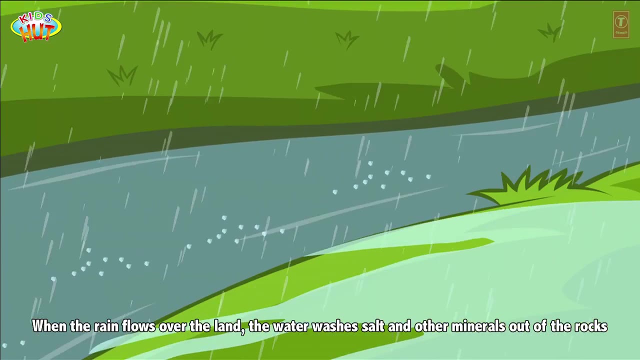 Yes, it certainly was, But Tia, why do I taste salt in my mouth? Why is the sea water salty? When the rain flows over the land, the water washes salt and other minerals out of the rocks and gets mixed with the water. 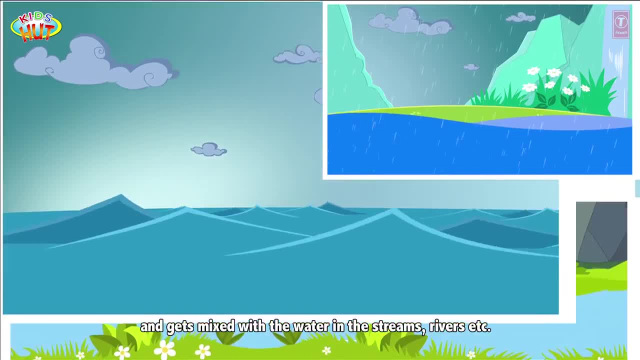 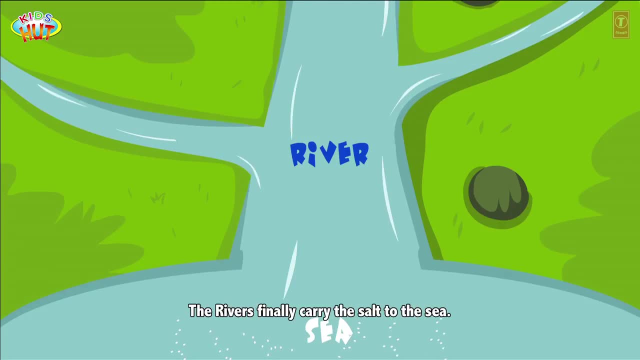 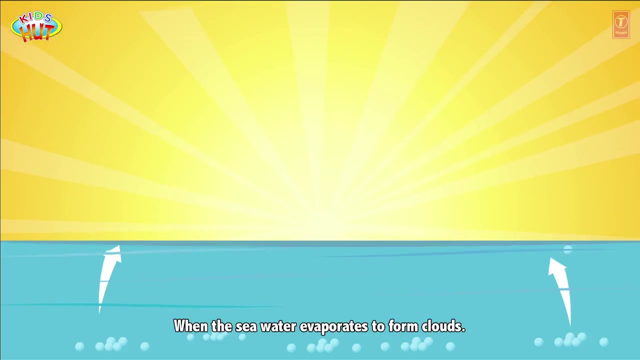 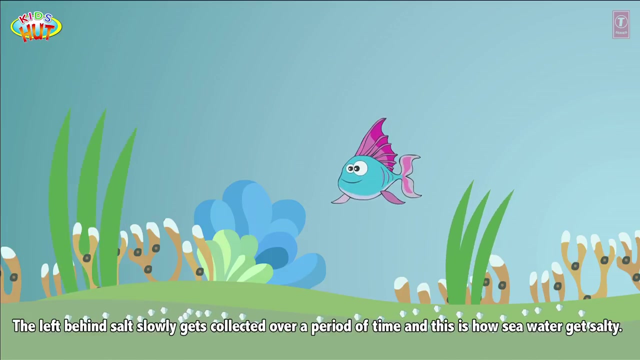 In the streams, rivers, etc. The rivers finally carry the salt to the sea. The salt stays in the sea as no water flows out of the sea. When the sea water evaporates to form clouds, almost all the salt stays behind. The left behind salt slowly gets collected over a period of time. 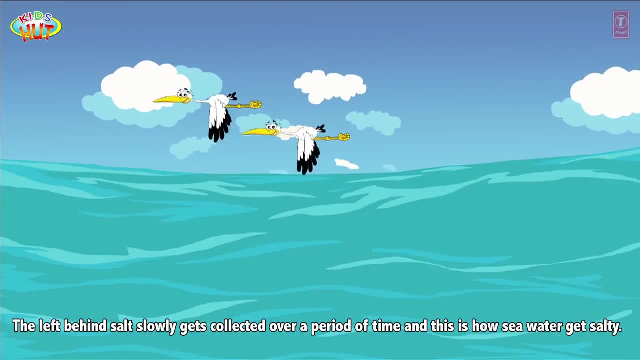 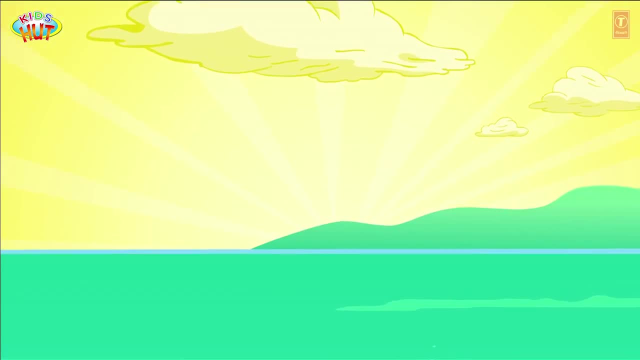 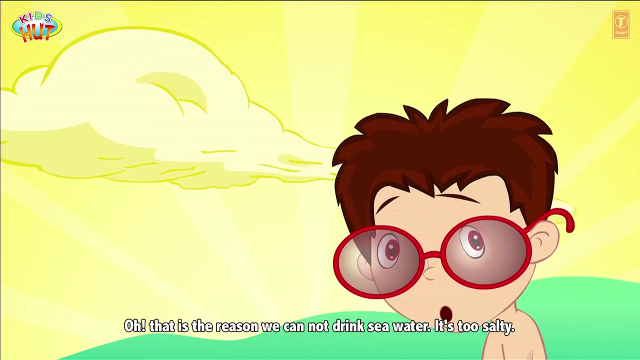 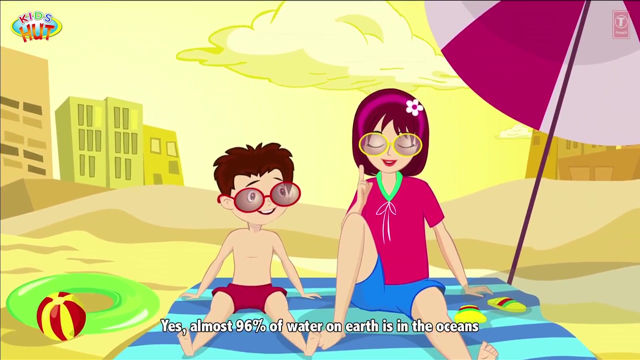 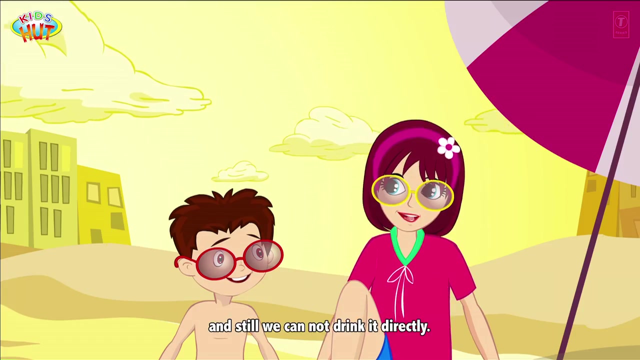 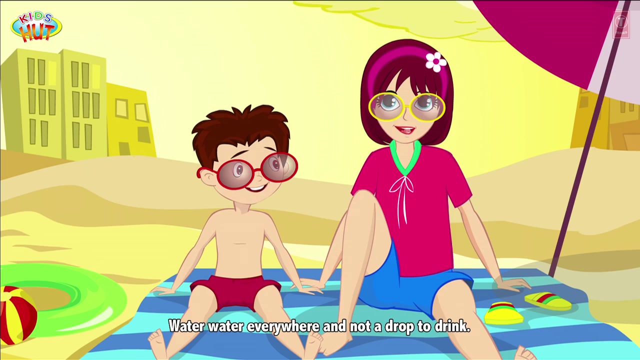 And this is how sea water gets salty. Oh, that is the reason we cannot drink sea water: It's too salty. Yes, almost 96% of water on earth is in the oceans And still we cannot drink it directly. Water, water everywhere and not a drop to drink. 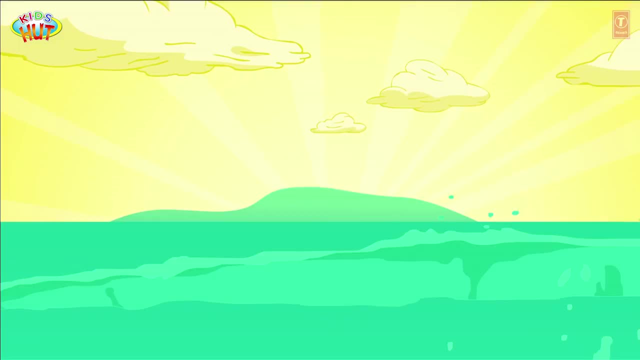 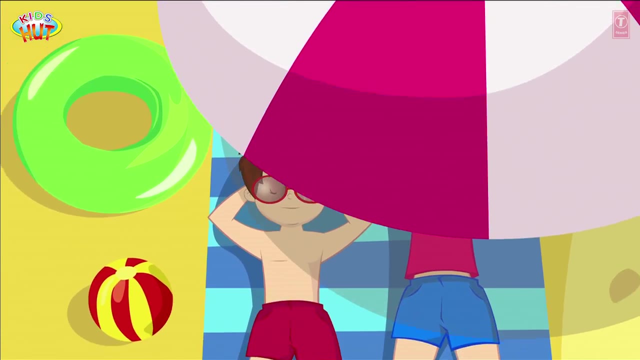 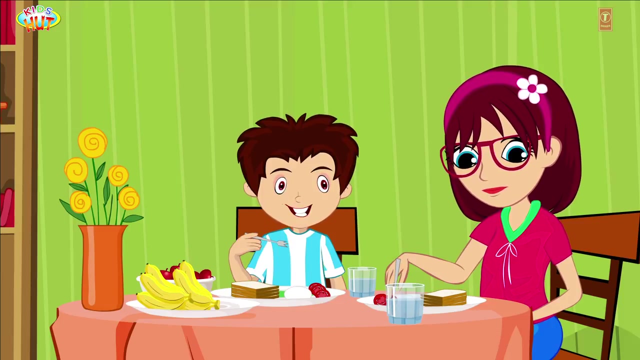 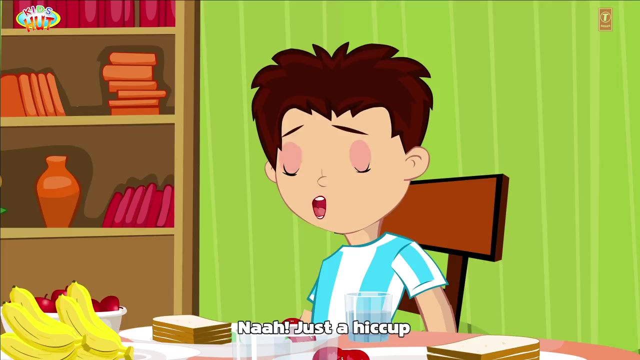 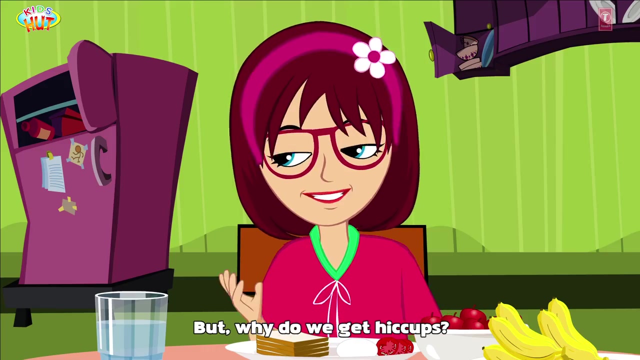 Ha ha ha. Tofu, are you alright? No, just a hiccup. But why do we get hiccups? Hiccups are funny ones. Most simple cases of hiccups come after eating or drinking too much or too quickly. 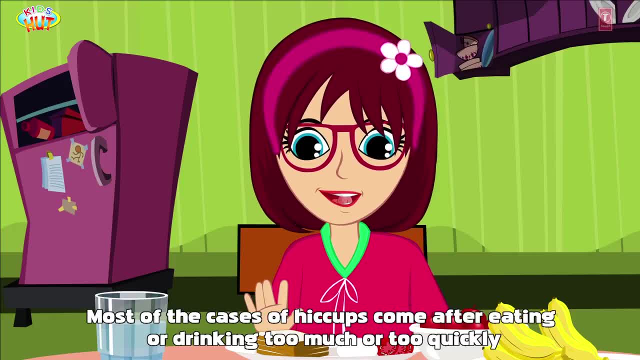 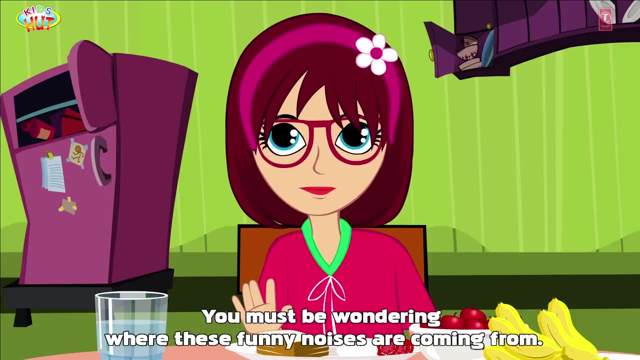 You must be wondering where these funny noises are coming from. The part to be blamed is the one that is not being heard. The hiccups are the ones that are being heard. The hiccups are the ones that are being heard. The hiccups are the ones that are being heard. 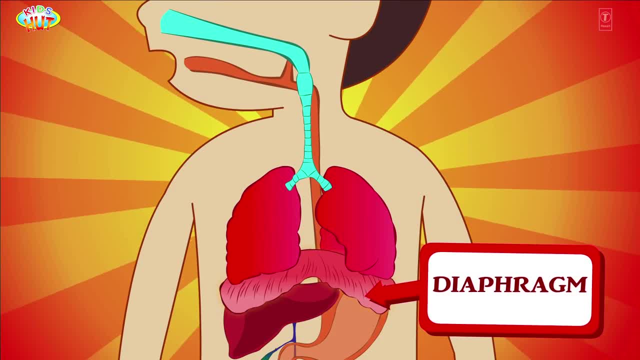 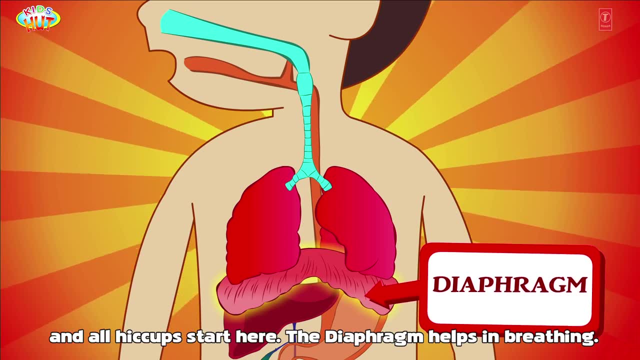 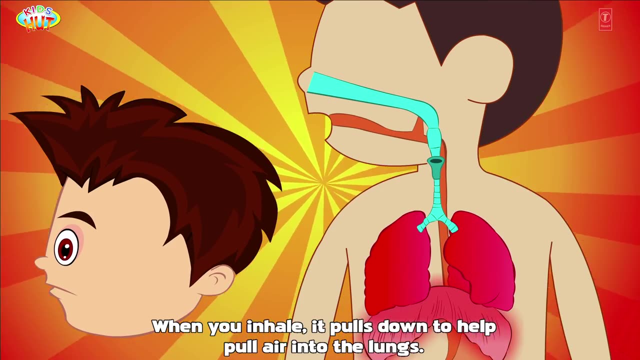 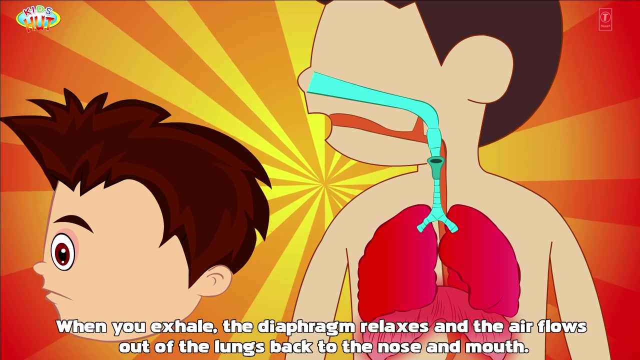 The first thing that is being blamed is your Diaphragm. This is a dome shaped muscle at the bottom of your chest, And all hiccups start here. The diaphragm helps in breathing. When you inhale, it pulls down to help pull air into the lungs. 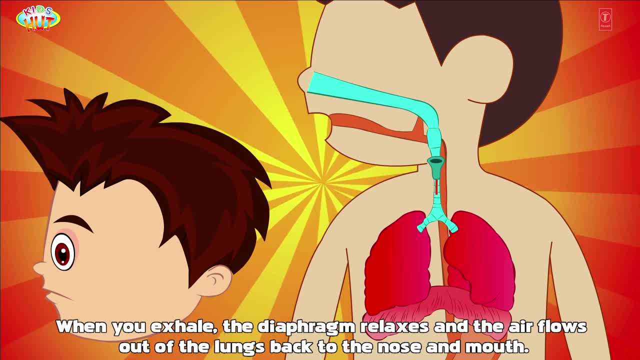 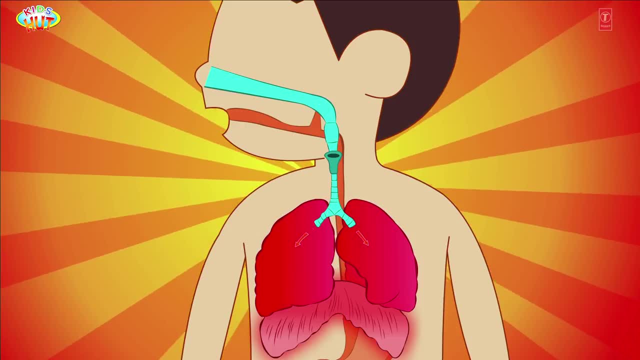 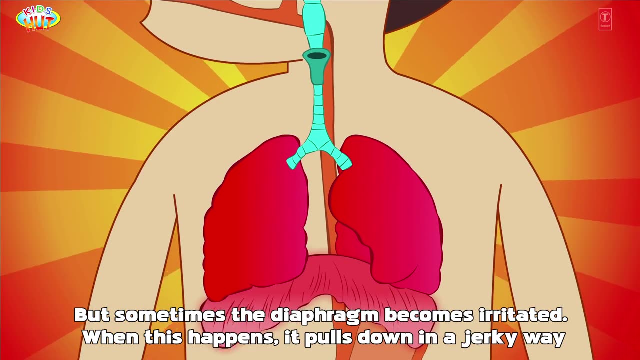 When you exhale, the diaphragm relaxes and the air flows out of the lungs to the stomach, Like this, of the lungs back to the nose and mouth. But sometimes the diaphragm becomes irritated. When this happens, it pulls down in a jerky way. 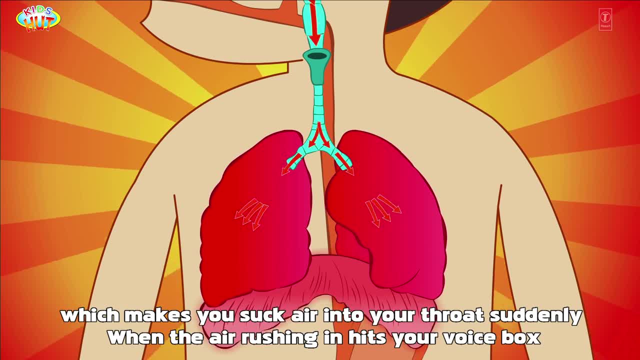 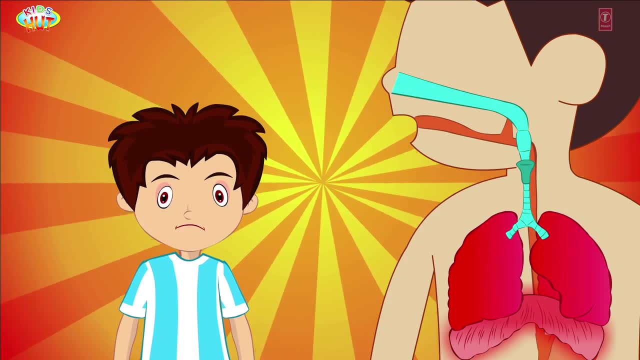 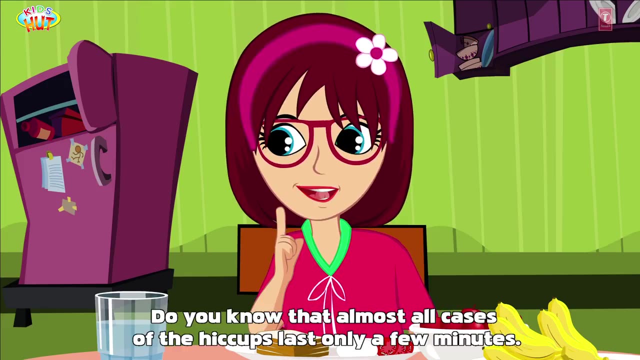 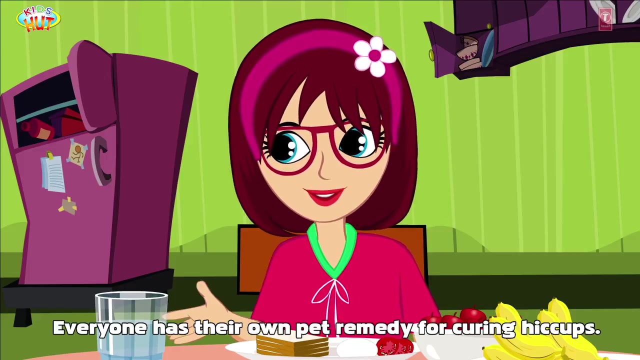 which makes you suck air into your throat. suddenly, When the air rushing in hits your voice box, you are left with a big hiccup. Do you know that almost all cases of hiccups last only a few minutes? Everyone has their own pet remedy for curing hiccups. 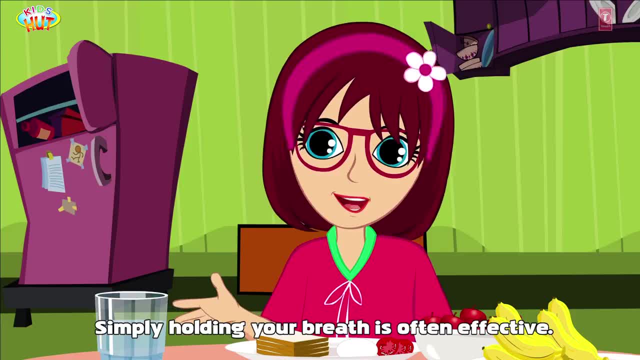 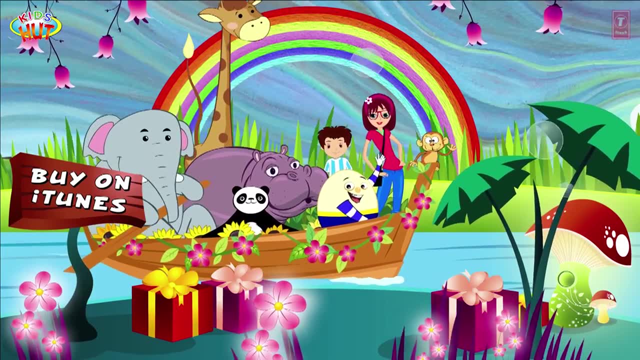 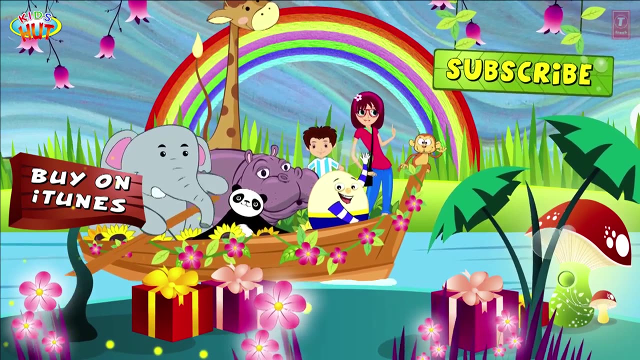 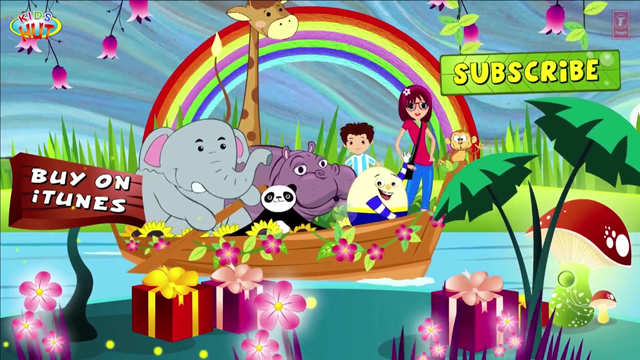 Simply holding your breath is often effective. If you want to know how to cure your hiccups, please visit our website at wwwdermatologistcom. wwwdermatologistcom.